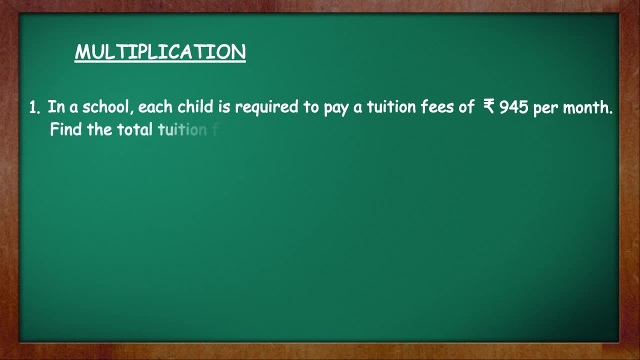 Per month. Find the total tuition fees paid by a student for 9 months. The fees for one month is Rs 945 and you have to find the fees for 9 months, for which we multiply 945 by 9.. Let's begin with the first statement. We know the fees for one month: Rs 945.. Now 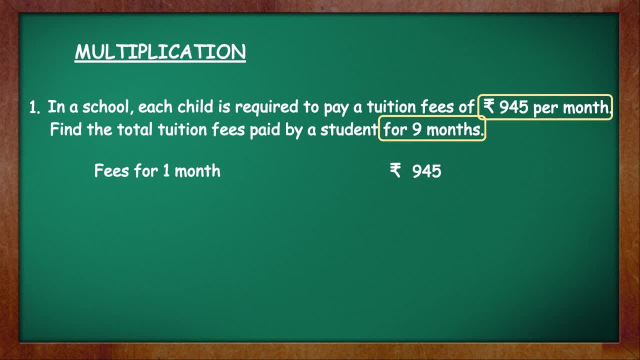 we can straight away find the fees for 9 months. So we write therefore fees for 9 months and to find that you have to multiply 945 into 9.. So write that multiplication statement, 945 into 9, and then do the multiplication below 945 into 9. when you multiply, the product is 8505.. Write the answer with the. 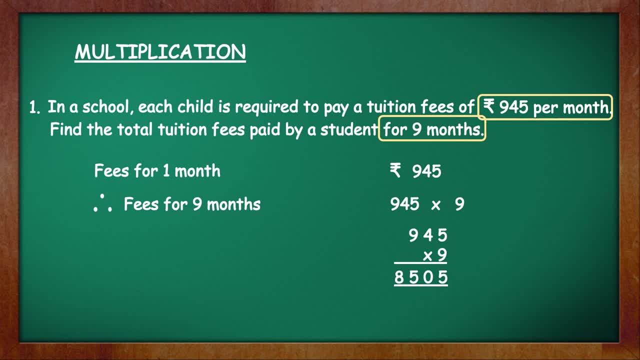 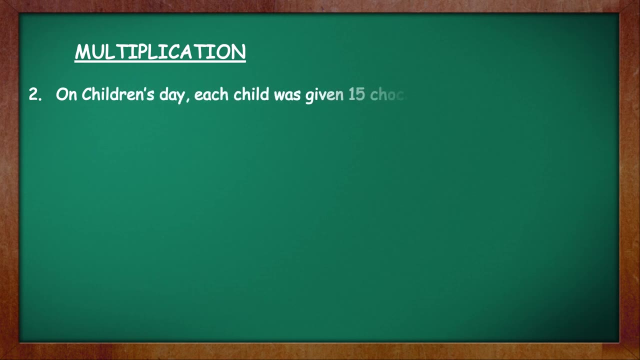 unit. The unit here is Rs, which is written before the number. So the answer is equal to Rs 8505.. Second question: On children's day, each child was given 15 chocolates. How many chocolates were given to 783 students Here? we know the number of chocolates given to each student. 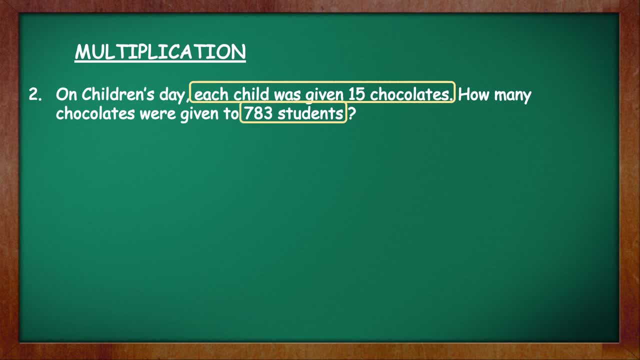 and we have to find out the number of chocolates given to each student and we have to find the number of chocolates given to 783 students. To find that, we have to multiply the number of students by the number of chocolates given to each student, That is, 783 into 15.. Begin. 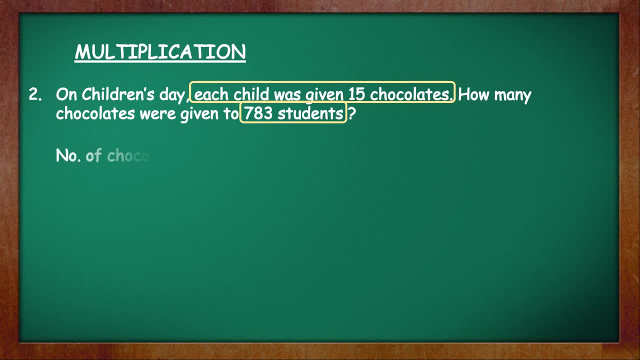 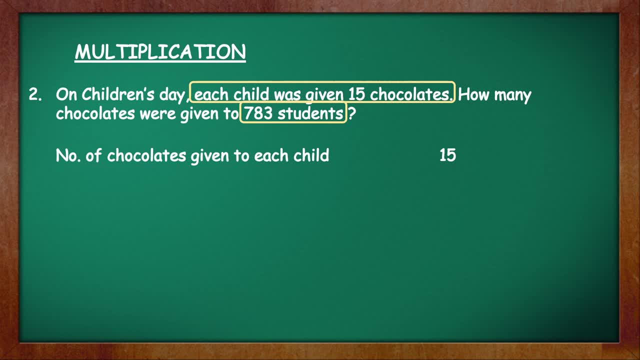 783 students. For that the statement is therefore number of chocolates given to 783 students. and to find that we have to multiply 783 into 15.. So write that multiplication statement first and then solve it below 783 into 15.. We'll do long multiplication here. First, multiply by 5.. 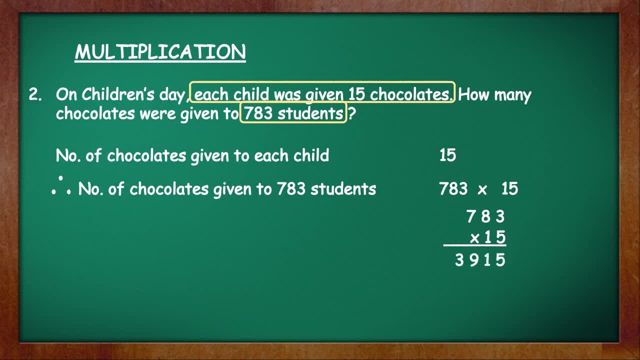 783 into 5 is 3915.. Next put the 0 and multiply by 1.. 783 into 1 is 783.. Then add both the numbers, 11,745.. That is the total number of chocolates given to 783 students. Answer is equal to 11,745 and the 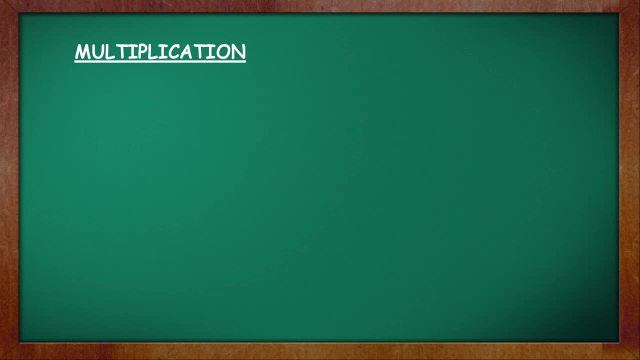 unit is chocolates. Question number 3.. In a school there are 2,345 students each in the primary, middle, senior and senior secondary sections respectively. How many students are there respectively In this question? we know the number of students in each section and the different sections are. 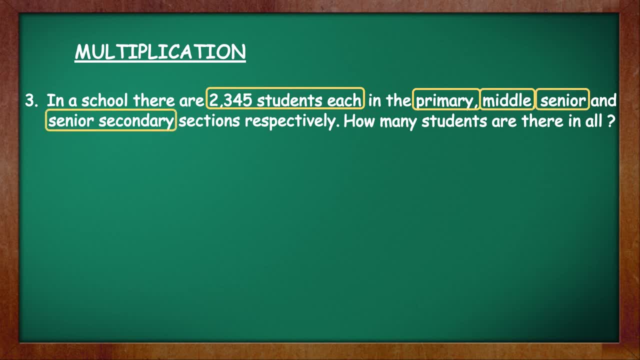 primary, middle, senior and senior secondary. That is 4 sections in all. In order to find the total number of students, we have to multiply the number of students in each section by the number of sections. Let's begin. First statement is number of students in each section: 2300. 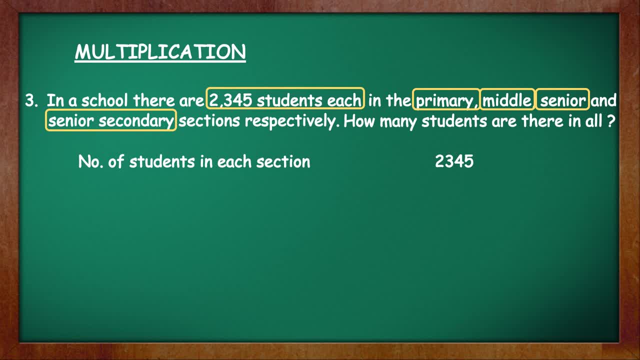 Next we'll write the number of sections, as that number has not been given in the question. Only the different sections have been named, So we will write number of sections, which is 4.. Now we can find the answer. So write, therefore, number of students in all, and to get that we have. 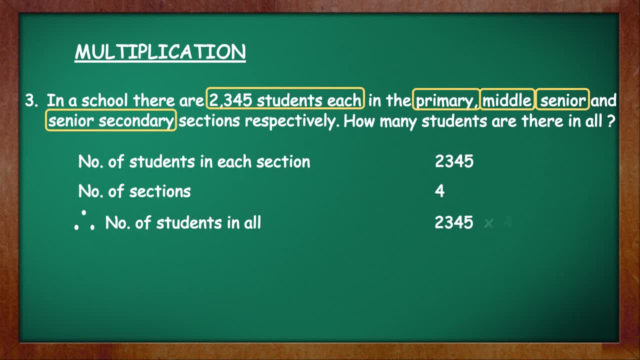 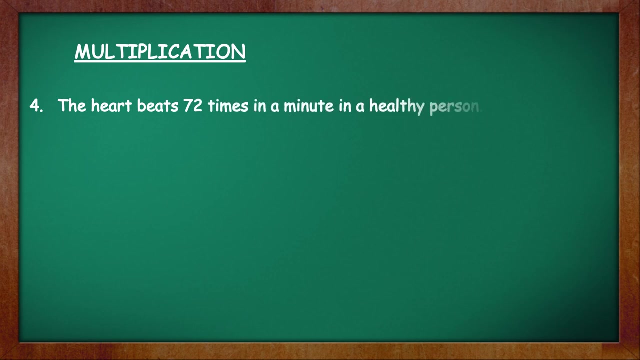 to multiply 2345 into 4.. Write that multiplication statement And multiply below 2345 into 4 is equal to 9380.. Answer is equal to 9380 and the unit is students. Question number 4.. The heart beats 72 times in a minute in a healthy person. How many times will it beat in an hour? 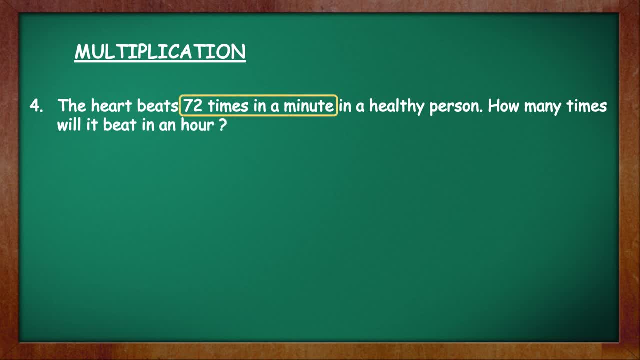 Here. we know that the heart beats 72 times in a minute in a healthy person. So how many times will it beat in an hour? the number of times the heart beats in a minute. but we have to calculate the number of times it will beat in an hour. so before we begin the calculation, we have to convert this r into: 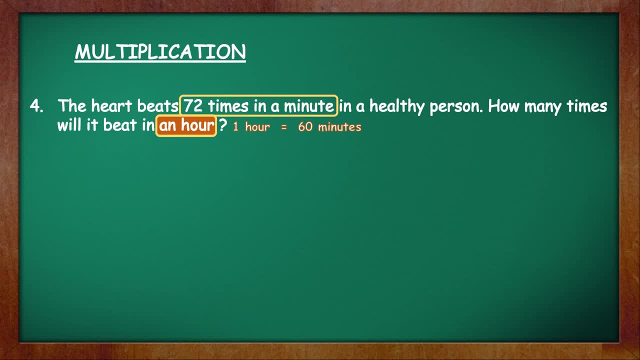 minutes. let's begin with the first statement: number of times heart beats in a minute: 72. next, write the number of minutes in one hour, which is 60.. after this we can calculate the answer. so write the statement, therefore: number of times heart beats in an hour. and to know that, what must. 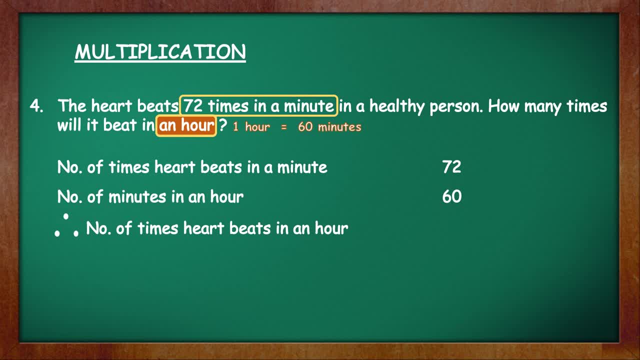 we write the numbers that have to be multiplied 72 into 60.. here we can use our knowledge of multiplication by multiples of 10, as 60 is a multiple of 10.. write 0 and then multiply 72 into 6 is equal to 432.. 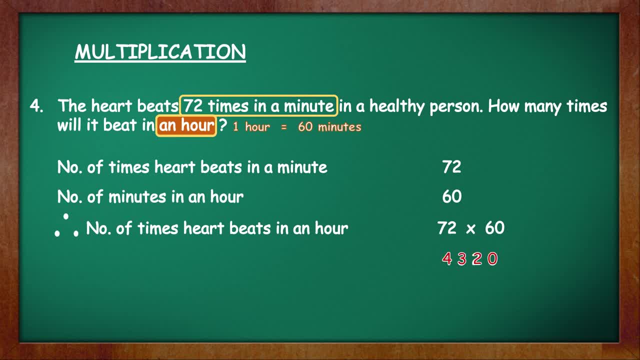 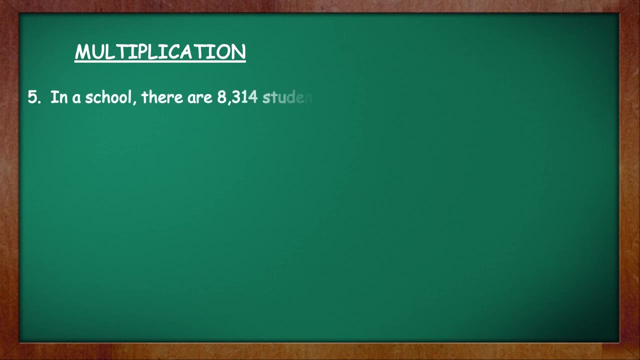 the answer is 4320.. write the answer with the unit: 4320 times. the heart beats in an hour. question number five: in a school there are 8314 students. if each child is given four library books to read, how many books were distributed among the students in this question? we know the total number of. 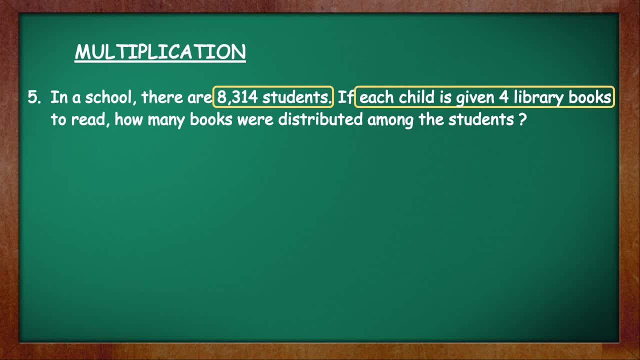 and the number of library books given to each student. in order to calculate the number of books distributed, we have to multiply the number of students by the number of library books given to each student. so let's begin. first write the number of students- 8314- then the number of books. 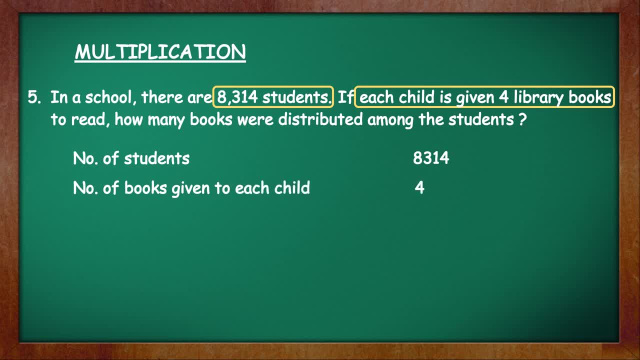 given to each child four. after that we can calculate the answer, therefore. number of books: 8314 into 4. remember it is important to write both the numbers that have to be multiplied after the last statement and then do the multiplication below. 8314 into 4 is equal to. 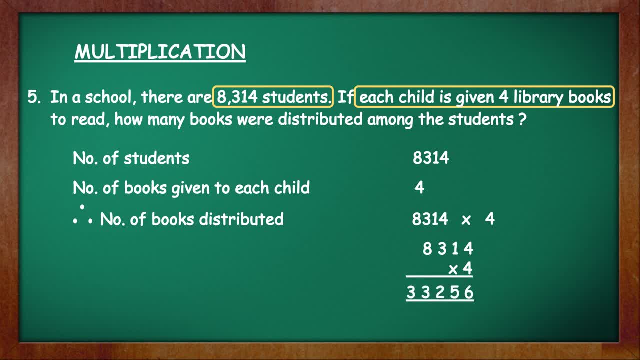 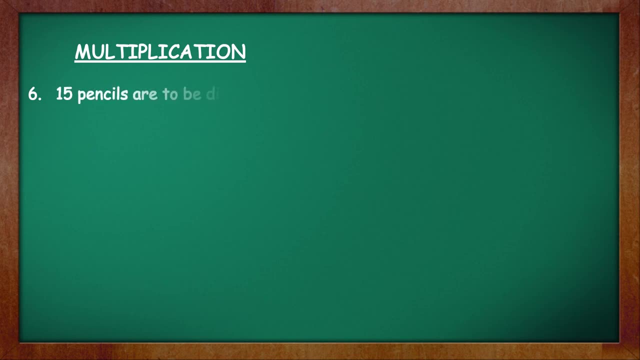 33 256. the answer is equal to 33 256 and the unit is books 336.. just like the number of children we have, prepare the number of books that we write three separate cases here. if the number of children is GET, then P spend. that is equal to. 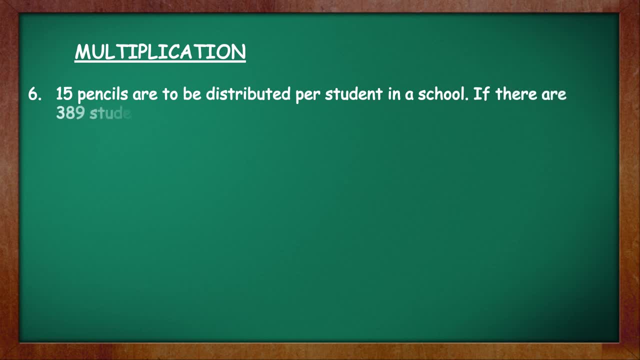 33ả haqq". alright, we solved till the last question. one last question before we end: 15 pencils are to be distributed per student in a school. if there are 389 students in the school, how many pencils are required in all? 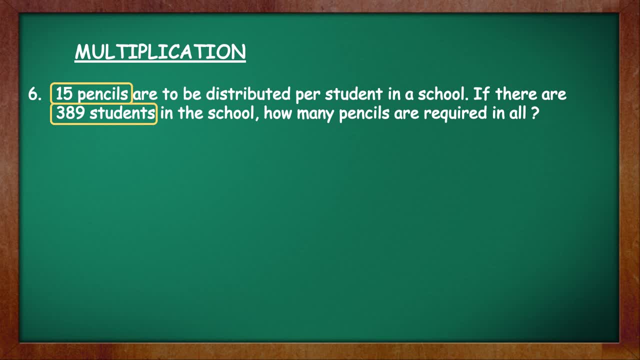 we know the number of pencils given per student and we know the total number of students. in order to find the number of pencils required in alld pencils given per student, begin with the first statement- number of pencils distributed per student, which is 15. then write the number of students, which is 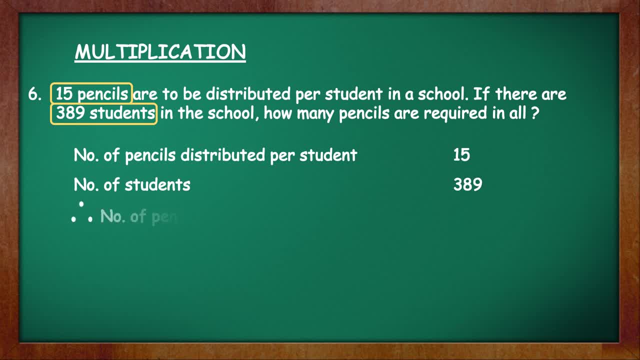 389. therefore number of pencils required will be 389 into 15. arrange the numbers for the multiplication: 389 multiplied by 15, we'll do long multiplication here. 389 into 5 is 1945. then write 0 and multiply by 1. 389 into 1 is 389. and when? 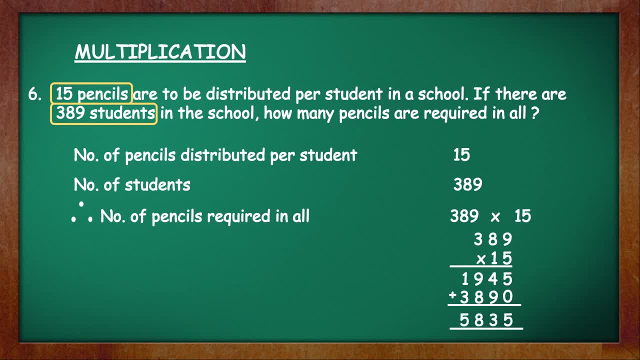 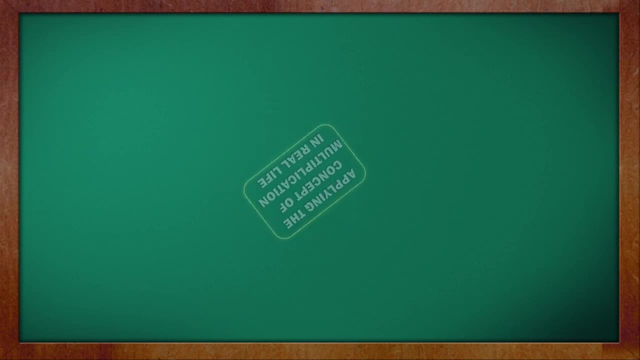 we add both the numbers, we get 5835. the answer is 5835 and the unit is pencils you.